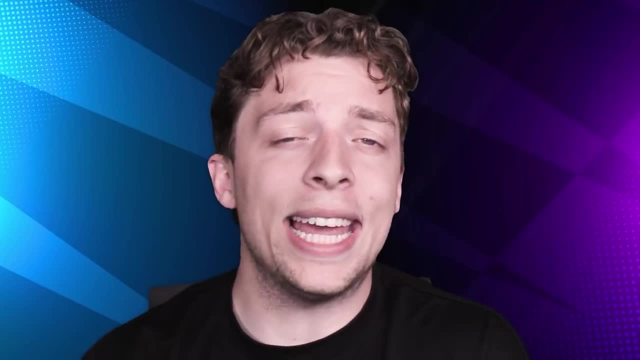 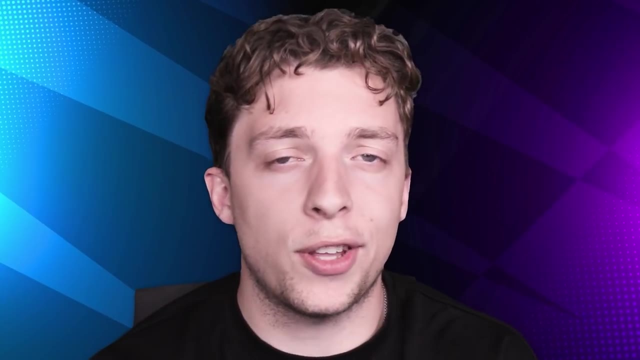 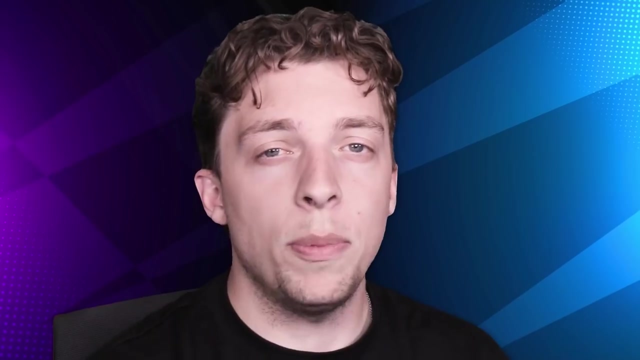 Thanks to Gamers Without Borders for sponsoring this video. This weekend, I'll be participating in the second edition of the biggest charity esports festival in the world. Gamers Without Borders is donating the total of 10 million dollars to charities issuing COVID vaccinations to developing countries. I'll be joining the Rocket League show match with the $50,000 prize. 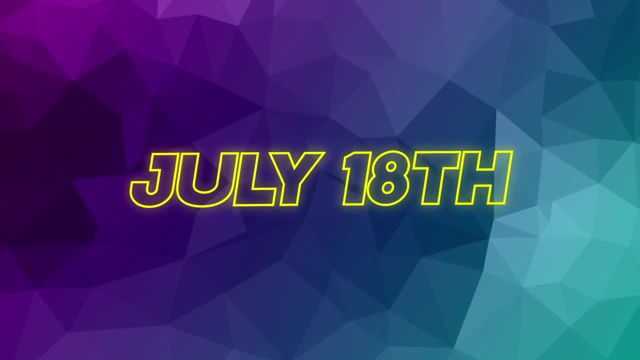 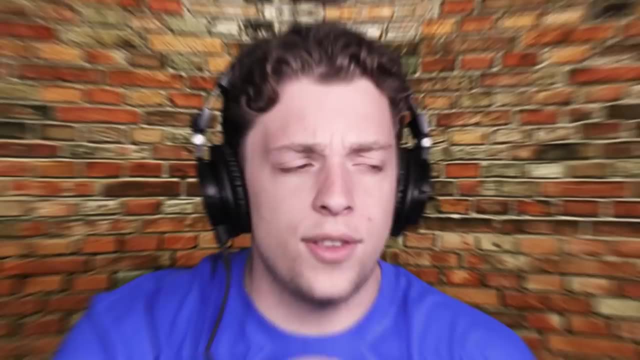 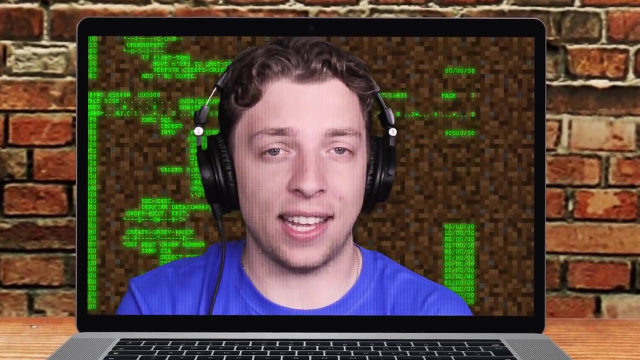 pool going to charities. The match will be taking place on July 18th at 4: 30 pm BST. Make sure to watch the match live and check out GWB at the links in the description. So long story short. we installed a mod that makes Minecraft extra realistic by adding real physics to the game. So 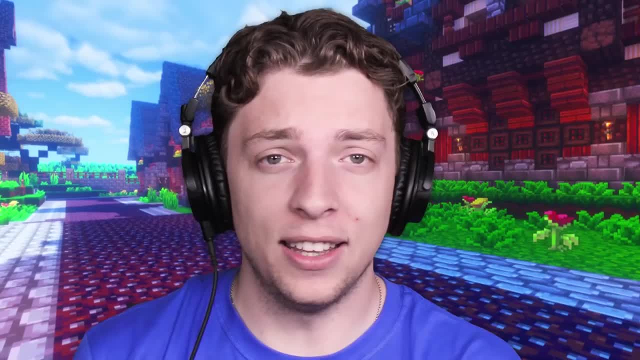 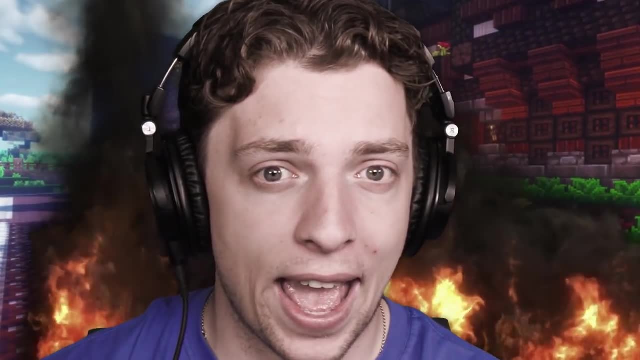 you know trees, where you cut them down, they just sort of float. That doesn't happen today In this video. it all collapses. But one thing I will say is the video kind of goes off the rails a bit. so yeah, I'm not going to say anything more than that. but what I will say is I'm wearing the Super. 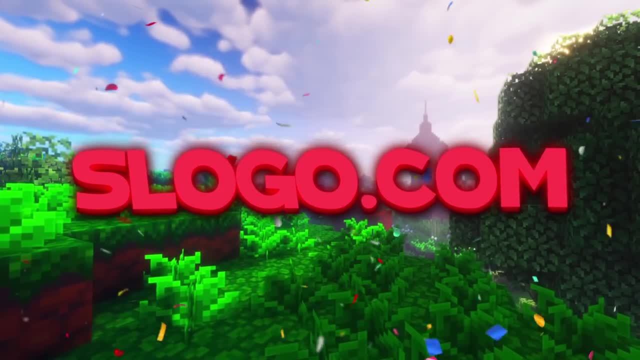 Slug t-shirt, which is sold out. But hey, you guys, check out the Sluggercom. maybe we'll bring it back soon. Click the like button if you want to see it again And let's get into the video. Whoa, This is realistic. 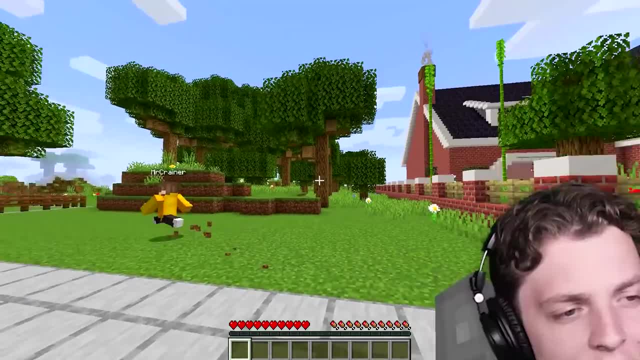 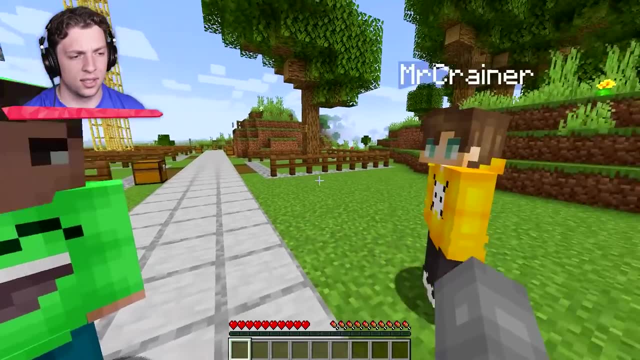 What, What That Guys? come on, come on. This looks like something you know about Minecraft. This is just Minecraft. What are you talking about? We're doing physics experiments in Minecraft, please, But, Jelly, there's no physics in Minecraft. 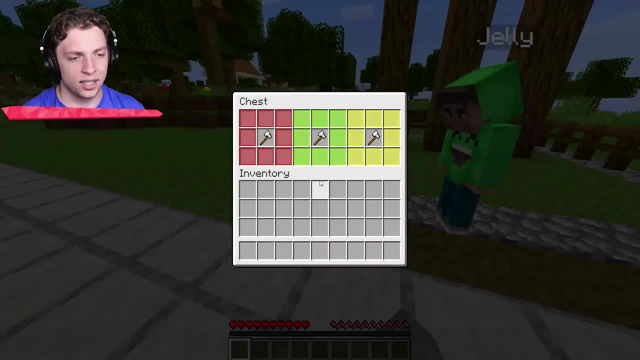 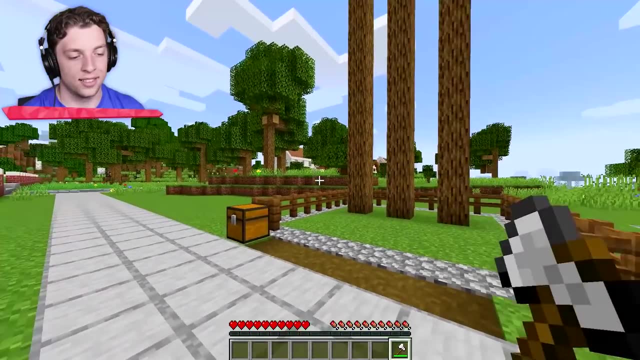 What are you talking about Jelly? That's the whole point. We have added them. Guys, look inside this chest you have an axe Craner. use the axe on the tree, Okay. Oh wait, that's you, Josh. don't on me. 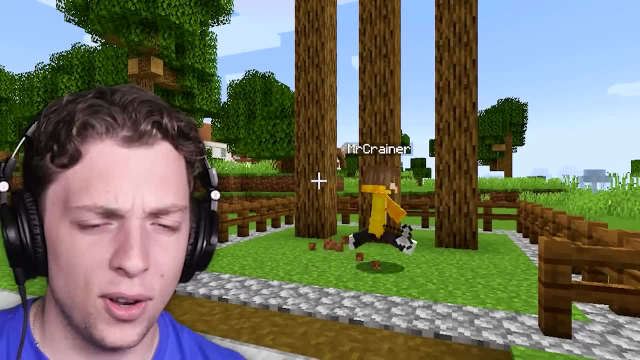 Do I look like a tree to you? I'll use it. I'll use it. I'll use it. okay, What are you doing? What are you doing? Watch this, it's going to be realistic. Whoa, Whoa. 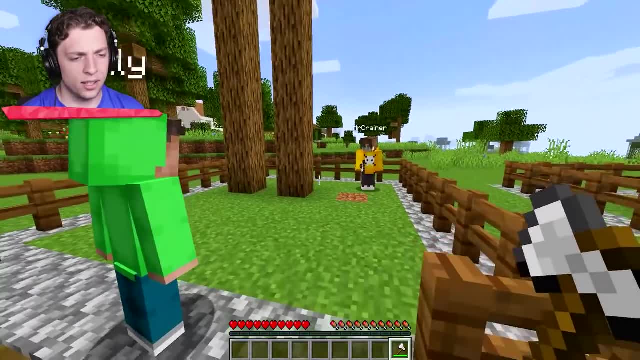 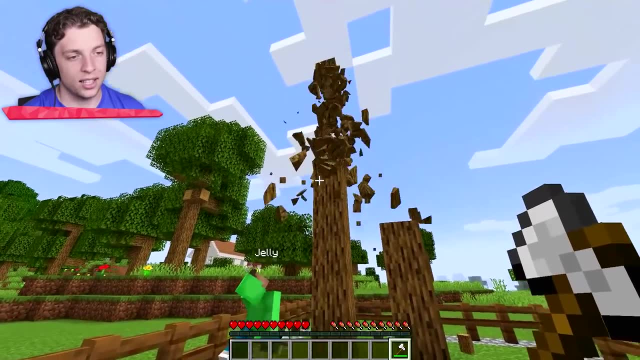 Did you see that? What Did you see that? Wait, Okay, that's actually insane. Wait, what if I do it from halfway up? Oh, What if I do it from all the way up? That wasn't all the way up, Jelly, That was about halfway still. 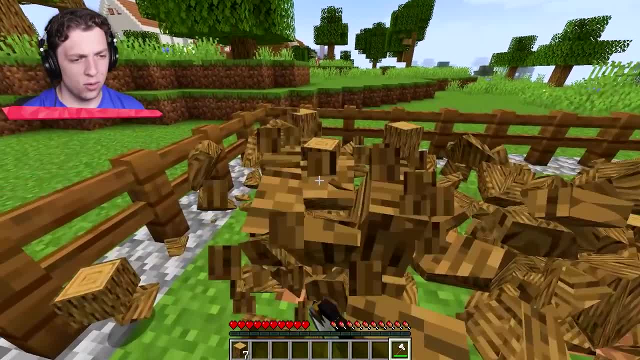 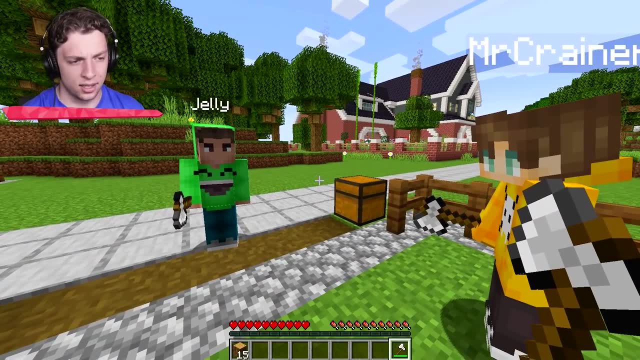 Dude, this is actually crazy. How did you do this Jelly? Wait, so is this a new update? Basically, what you do is you do x divided by y times z times 3.771.. 23!. There you go. 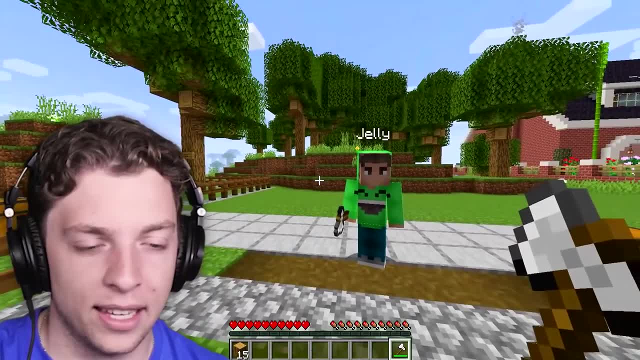 Crack the code That gives 23.. I just made the math. So how does that have anything to do with this? Physics, Josh? You won't understand. Yeah, you got physics, Josh, Experiments laying here, So what does this do? 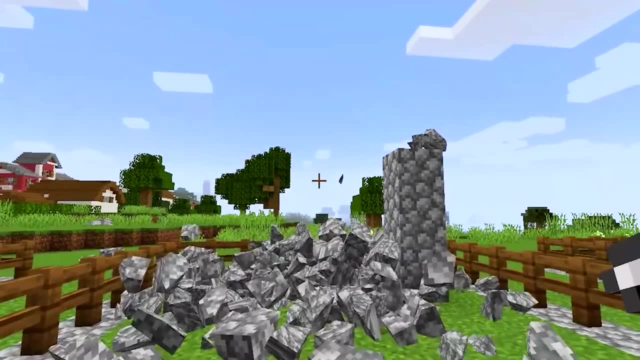 This one involves cobblestone. Oh my god, Jelly, you just missed it. You just missed that, I just missed it. Thank you, Josh. Well, you should be focusing a bit more. I can't, I can't do this. 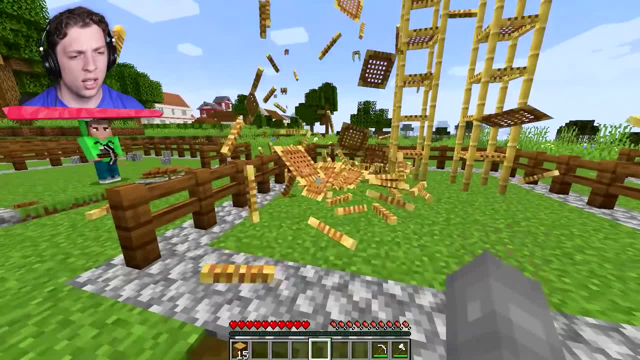 Okay, 3,, 2,, 1.. Wait, wait, wait, wait, wait, wait, wait. No, this is already, Josh. This is already Calm down. Um Gah, Hey, Hey, Jelly. 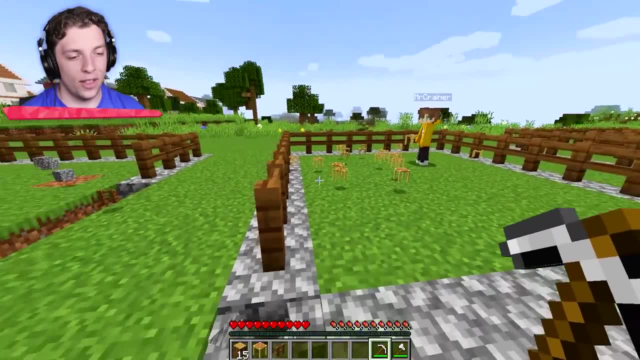 I hate to burst your bubble, but this already falls down. Normal Minecraft. Yeah, I don't know why that's there. I guess it looks a bit better. Crainer, put it down again. Put it down. Come on, stack it. 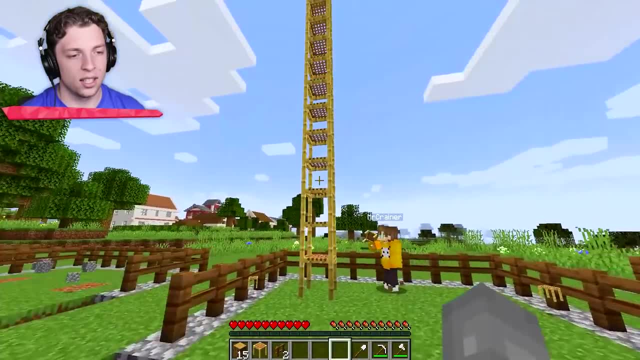 Wait. so what happens in here? Let me do it all the way up, Josh. don't ruin it. Don't ruin it, Josh. I know you want to, Don't ruin it. Hey, I just stole it. Look at that. 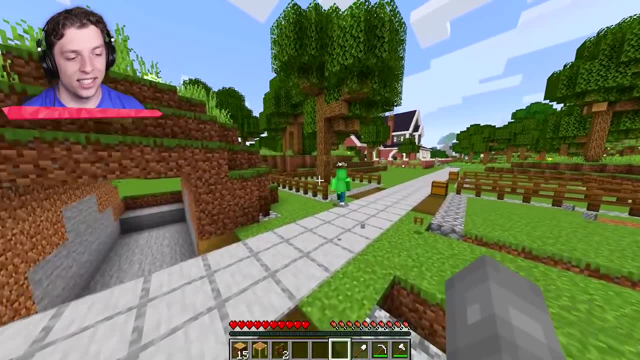 Jelly. why are you looking at me and not the thing? Okay, here's some rules, though, Josh. 3, 2, 1 before you do anything. okay, 3, 2, 1.. Josh, go ahead. 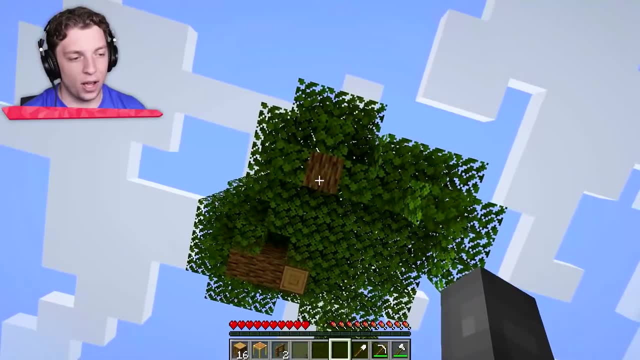 Okay, Whoa Wait. why did the ground break? Whoa Wait, it's still floating. It didn't even work all the way. Look at that wall. Oh my God, Get the last bit. We have more forest here, guys. 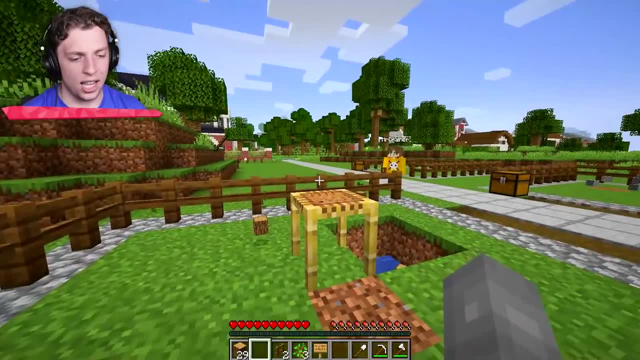 Come on, I can't get the last. Wait, I'm about to yell at you guys. Jelly 3, 2, 1.. Jelly and Josh, pay attention. Why did you have to count that down? Because I 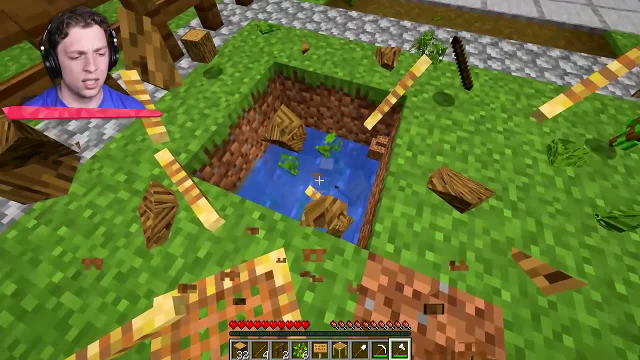 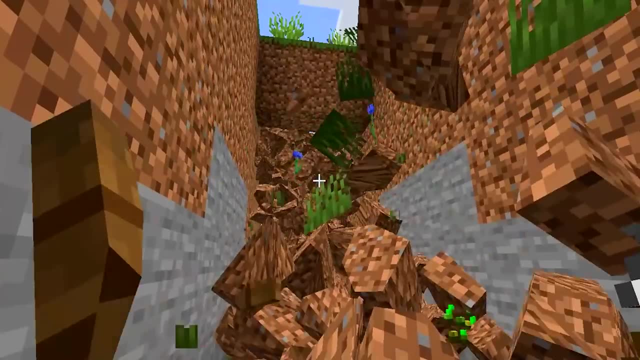 Warning. I gave you a warning. We actually need to stick together for this, because we all want to see the magic, okay, So stop being selfish, guys. I'm breaking this thing, Josh. you're doing not what I said- Whoa. 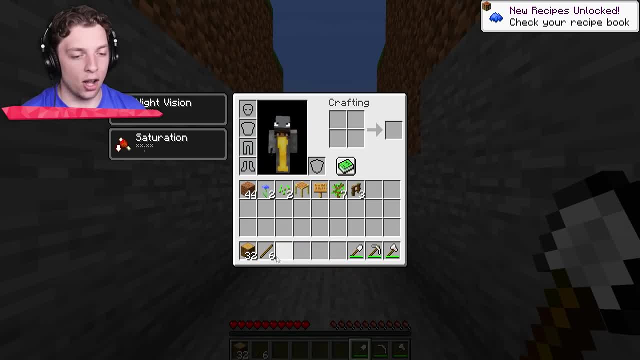 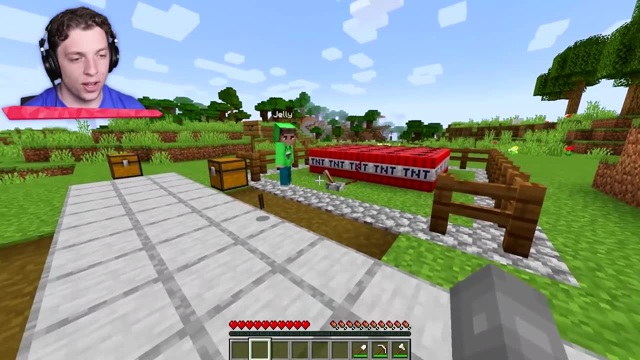 That's cool, right, guys? Yeah, Guys, look, I feel like there's a lot of anger going around right now and I feel like we should all just relax. What do you think? Can we please just Wait? I think we're supposed to do this first. 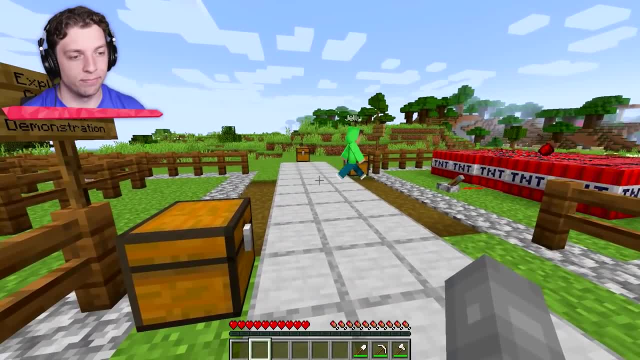 Kaboom time. No, no, no, We're supposed to do the creeper first Kaboom. Did you care about what we were supposed to do first? Josh, look, look, Look, Josh. Whoa, Whoa. 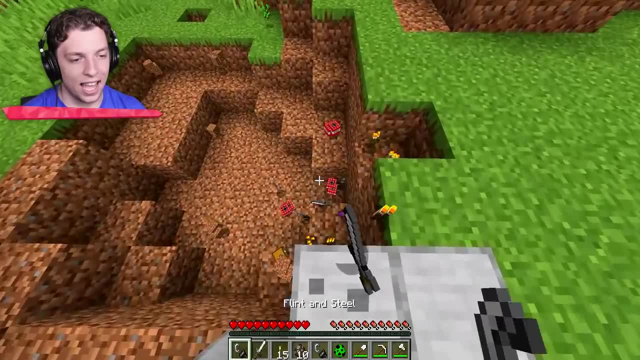 Whoa, Oh my God, Guys, you blew up the chest at the end. I want to do more of that. I want to do more of that one. I want to see That's the creeper. Yeah, you blew it up. 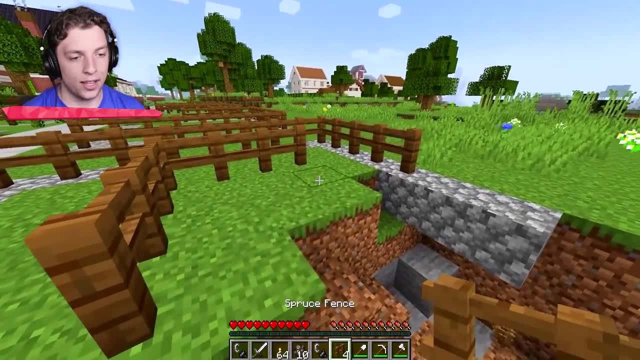 That was Jelly's idea. You guys took it out. No, You blew up the stuff in the chest. That was Jelly's idea, not mine, by the way. No, it wasn't my idea, It was Josh's idea. You said kaboom, and then I did it. 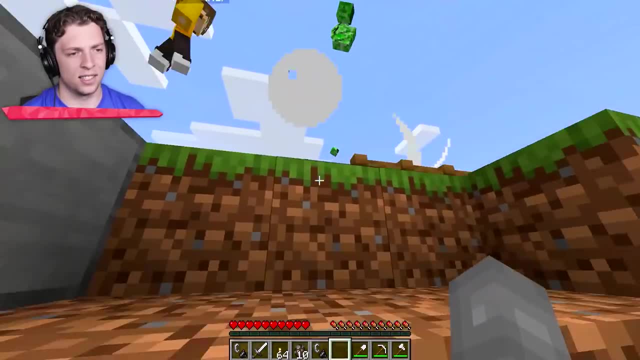 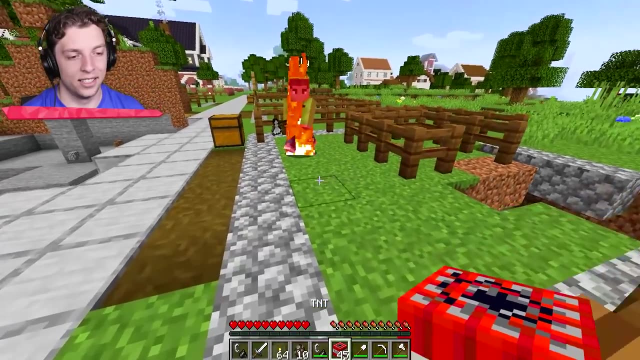 All right, What? Oh? he has the creeper. Oh, here we go. Hello, Yeah, yeah, yeah, Oh, the body part, Body parts. Josh, you were supposed to put the cow next to it. We are actually idiots. 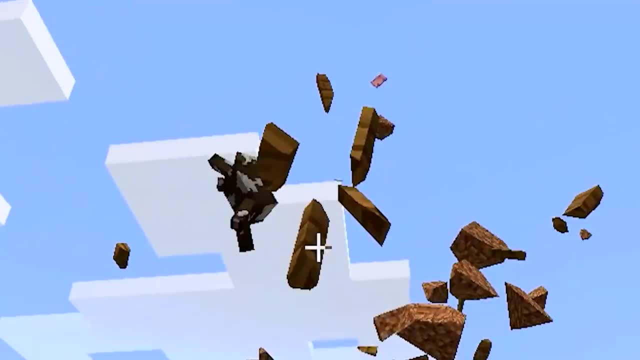 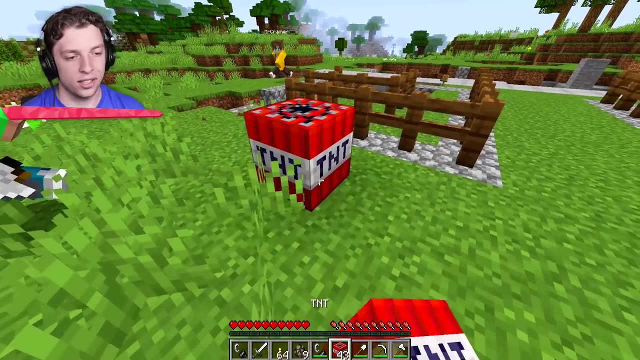 Oh, my God, Okay, Cow, Yeah. Oh, That was hilarious, Josh, Josh, Josh, Josh. Pretend you're the cow for a sec and put TNT again. I'll try to be the cow. I'll try to be the cow. 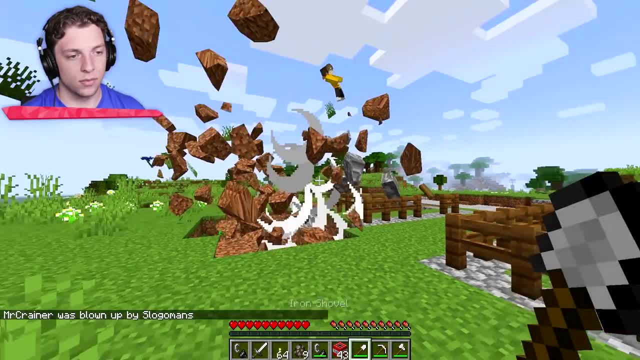 No, I don't want to be the cow. Craner can be the cow. Okay, Craner's the cow. Did it work? Hey, it worked. Did it work? Yeah, yeah, Wait, wait, wait. I didn't get to see it. 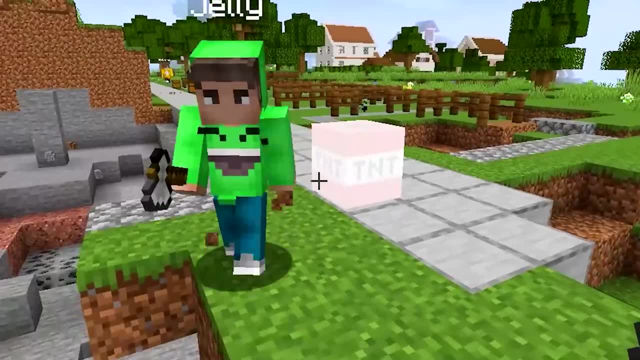 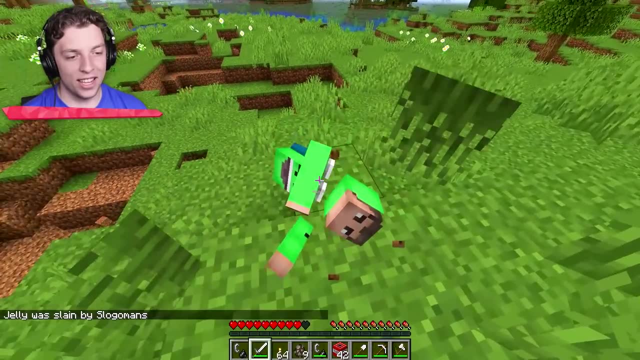 Can I please try it on somebody? Yeah, yeah, Jelly will do it. No, Jelly, no, I'm not even there. Josh Jelly's next, Just stab him honestly. No, Hey, Oh, my God, Wait, you can eat it after the fact. 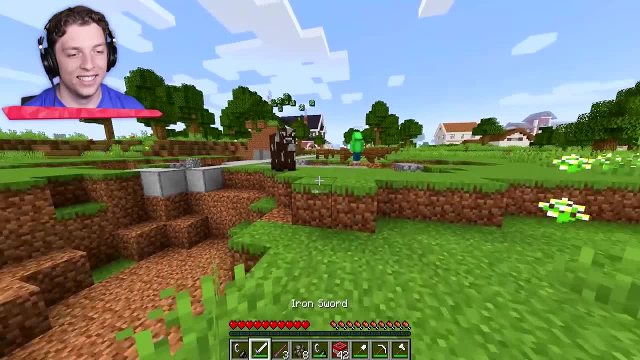 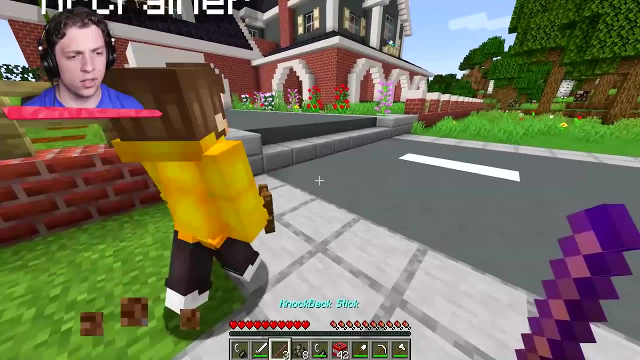 Josh, you need to stop. Josh, you need to stop. You're going to get banned, okay. Hey See, We all died. Okay, I have one more thing I need to see, but let me just get my TNT first. 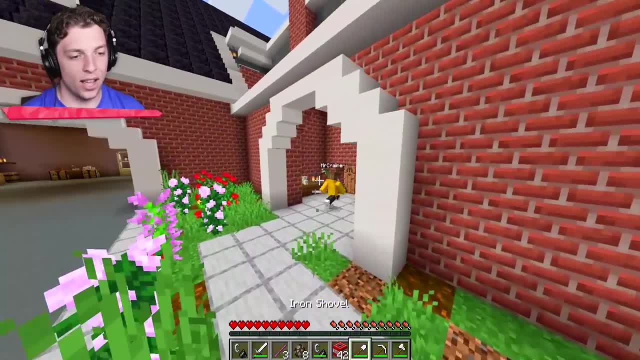 You don't have TNT in here. Where is it then, Craner? Yeah, there's TNT in the house. It's in here somewhere, Where. Where is it? Craner? Stop following me, because you're going to expose me. 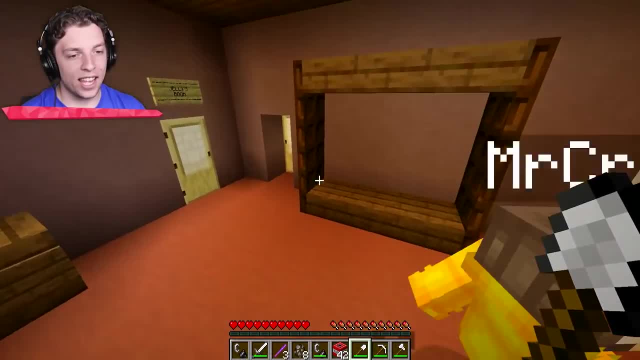 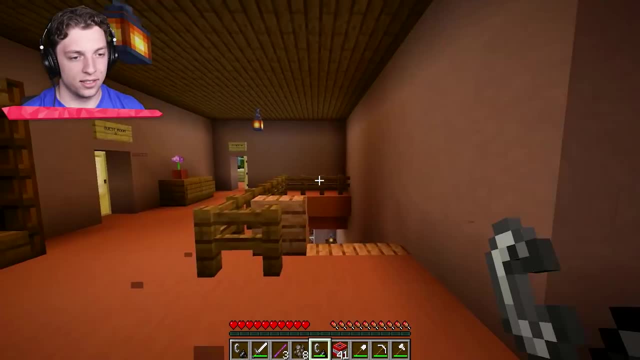 Where is the TNT Craner? You're going to expose me if you keep following me, Josh. Where's the TNT Craner? This is an unwritten rule. This says guest room one Craner Jelly. Yes, We need to have that petition now to ban Josh soon. 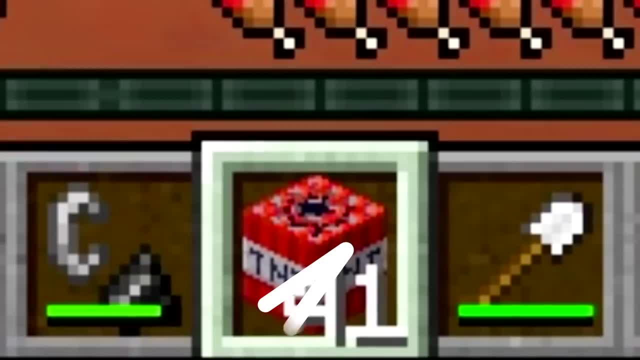 Okay, look guys, I'm going to be honest with you. I have all of the TNT at 45, okay, Okay, okay, Let's place it down around the house. Jelly, what are you doing, Josh? share one third. 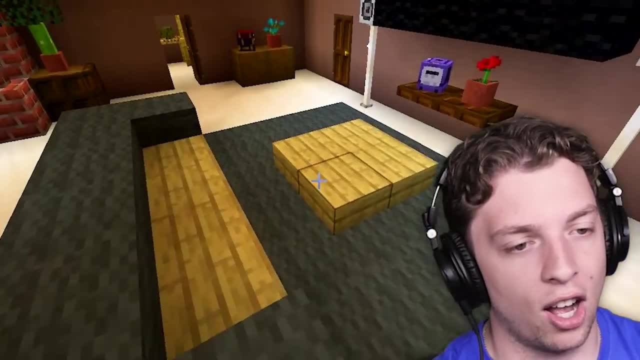 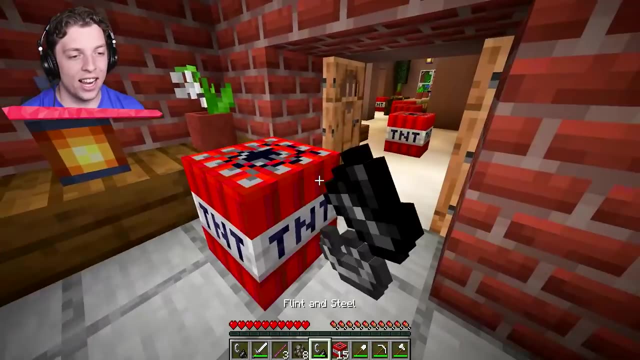 One. Yeah, All right, I'm going to set the charges inside of the house. Why is he the kid right now? He's supposed to be the clever one of us. Yeah, yeah, Josh. Yeah, yeah, yeah, All right. 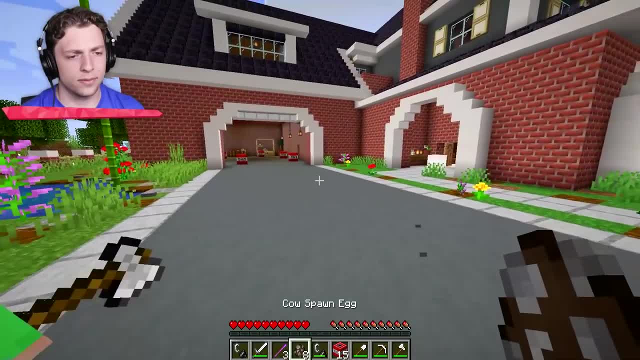 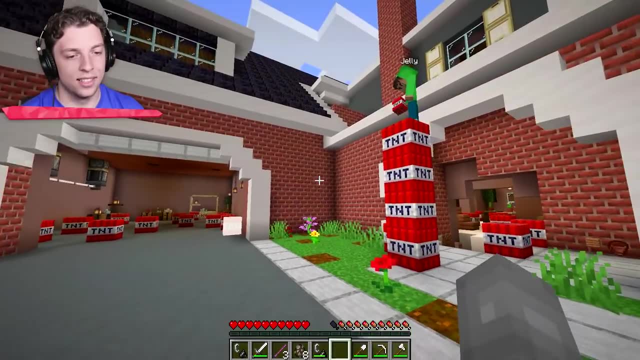 Why You're not living up to your expectations. Josh, I thought you were going to kill me Craner Kaboom house. That failed. Only one of them went off. Okay, Josh did it. He did it already. No, you're going to blow up the bottom floor Jelly. 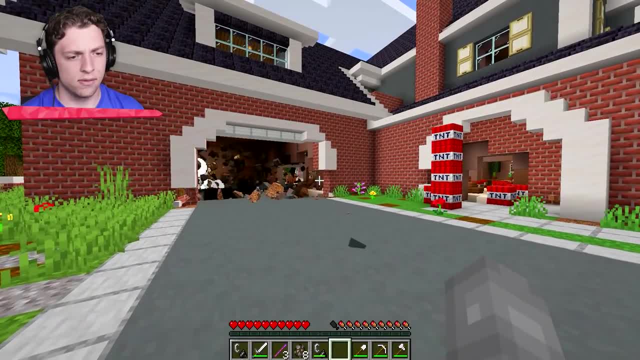 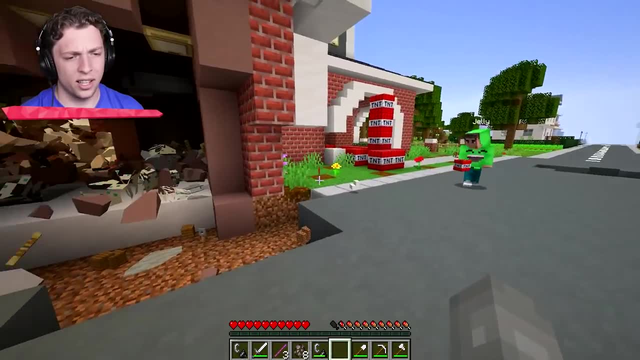 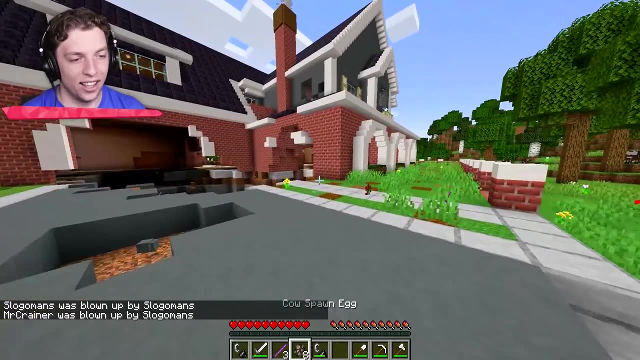 It's happening. Jelly, Oh my God, Oh, still going. Okay, Oh, Okay, Okay, This is amazing. Okay, I have an idea. We took this video for a turn. Let's just blow up stuff with TNT. 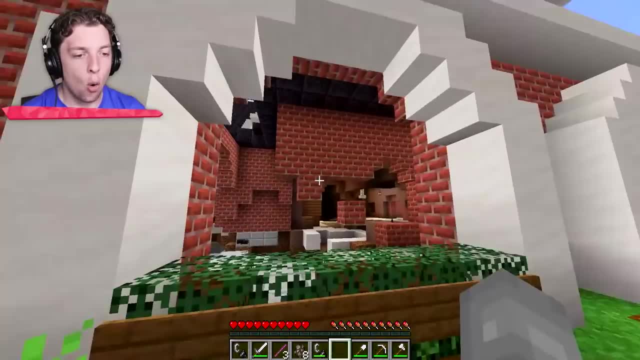 No, no, no, no, guys, I think first of all, we have to get rid of all of this, so the whole house collapses. So we need to break all of the connection points. Okay, Let's blow up the whole house. 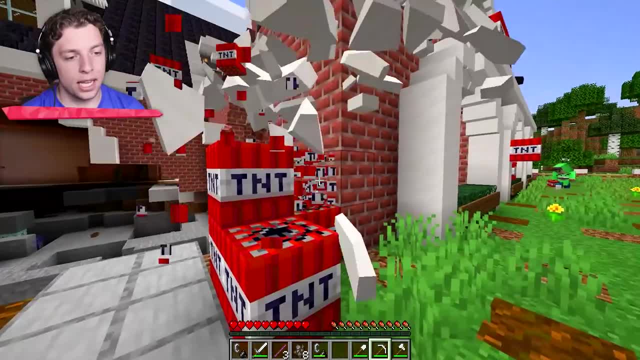 No, Jelly. don't go up Jelly Jelly. You missed it. You don't understand me. Blow up whole house. Blow up whole house Jelly, do you? Yeah, we need to blow up all the walls around it. 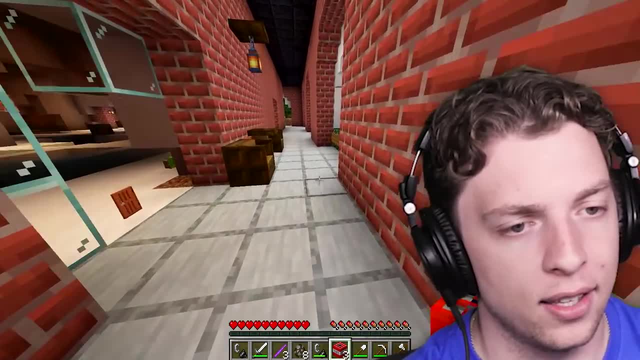 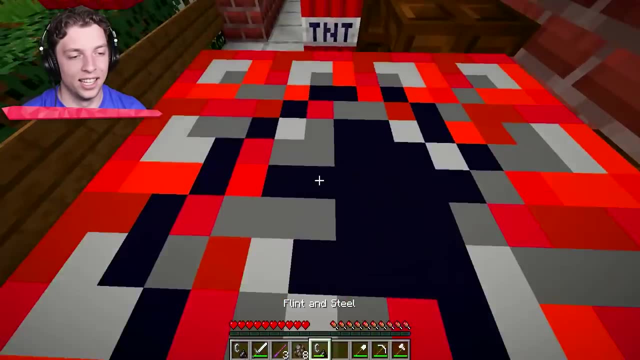 Josh, I understand, But you built up. You do not understand. The crazy thing is, we're all above 20 here, Josh. why, Why, Josh? Why do you keep disappointing me? I hate Josh and everything about him. What is going on with you today, Josh? 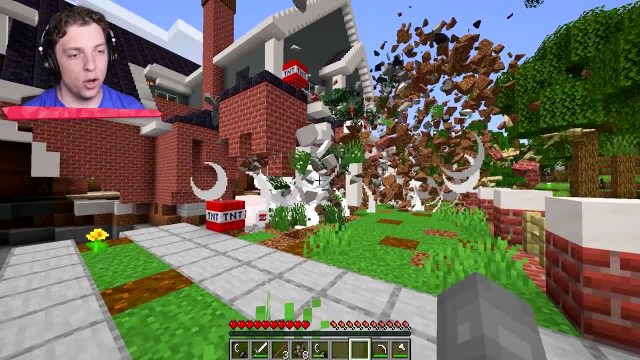 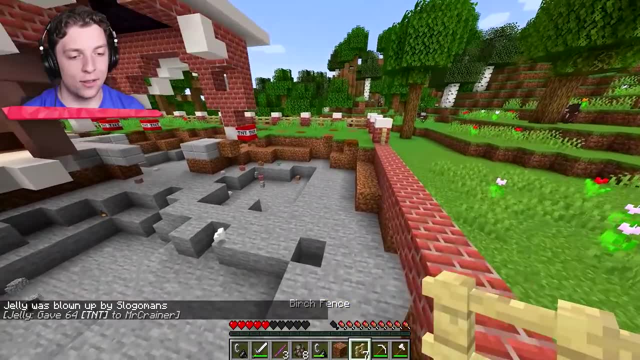 You guys are really bad at doing it. Am I Who keeps placing it high up? How did you die? What, Look guys, we're trying to break the bottom of the walls so it collapses. Do you understand? Why are we supposed to listen to you now when you don't listen to us? 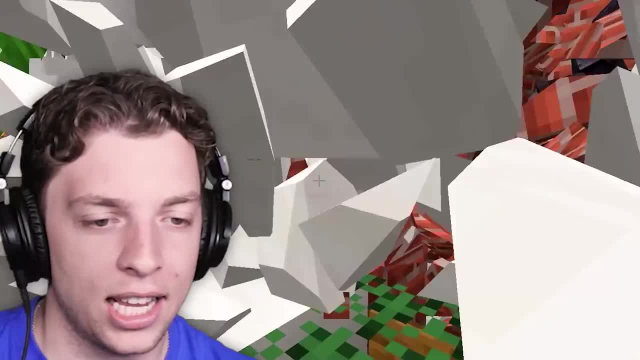 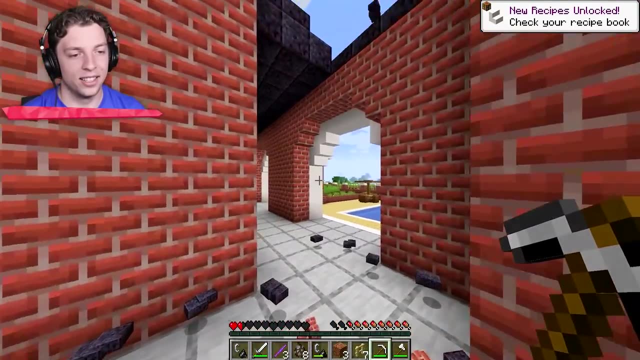 If you Look, I just like explosions. Josh, what did you do this morning? What, What different, What different. This is indeed, Josh. you know, this is weird for us, right With you, Josh. Josh, we don't know how to record when you're the one out of control. 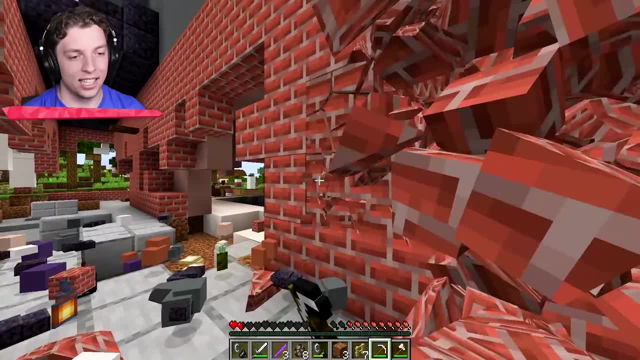 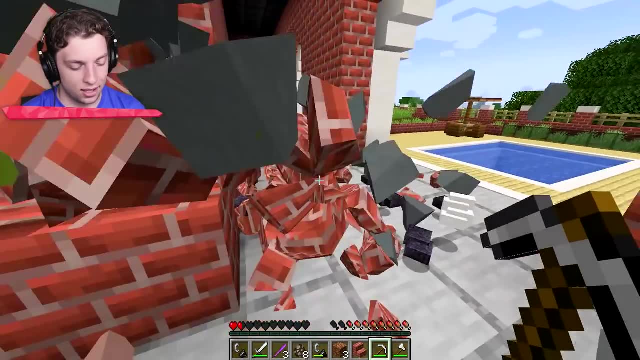 Look guys, we break house. Okay, house break, Josh. I actually feel uncomfortable. House break. I'm also uncomfortable. This is: Oh my God, I need more TNT Jelly. I feel like we just Need more TNT. 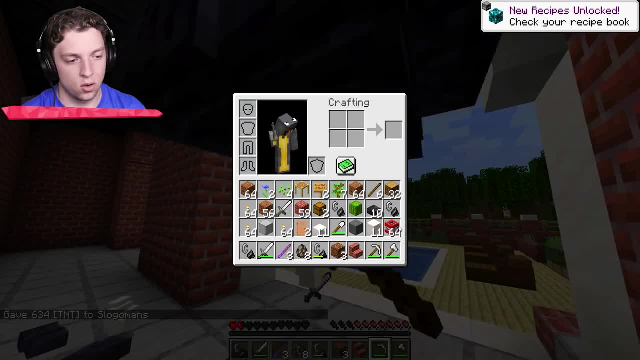 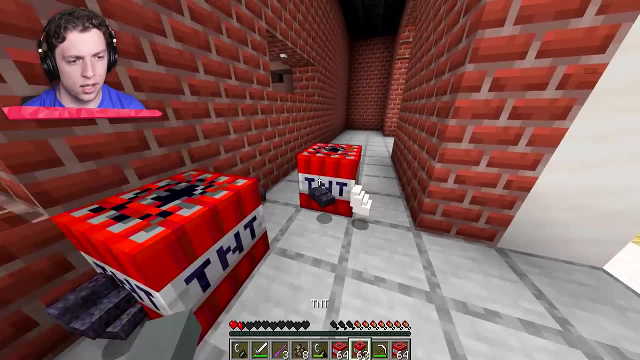 I need more. I don't know what to do, Jelly, I have an idea. You just let's sit by the pool and watch Josh unfold: More TNT. I feel like he's got another like a lot of idea, a lot of anger right now from recording. 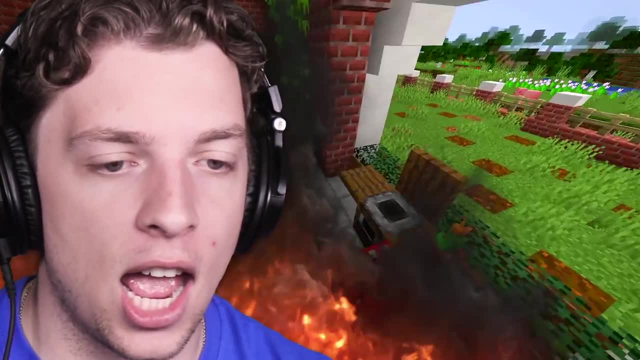 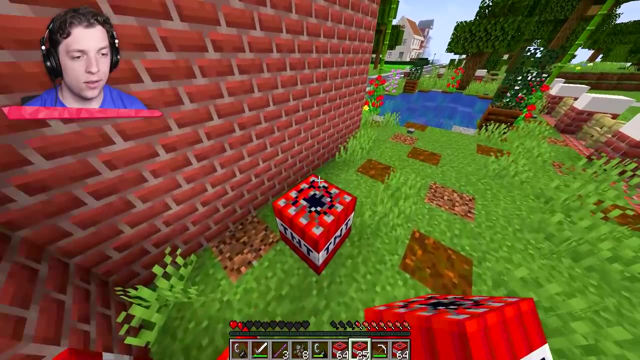 with us and he's letting it go now, More TNT. This is good for him. I think Jelly, this is Skeleton- be gone. Okay, This house will die. I feel like this is good for our friend Jelly. 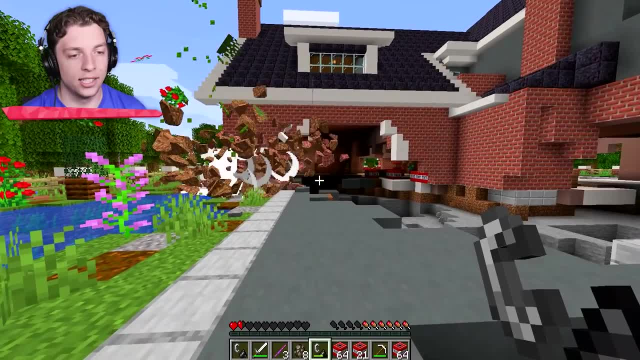 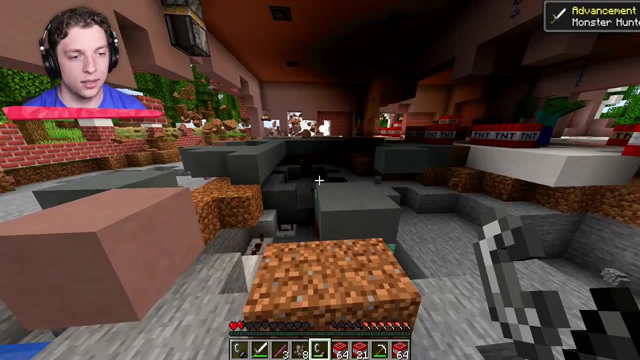 We should just let him More, More. Josh needs to steam up. Die house, Die. We're just letting this happen at this point, Jelly. We're letting it happen More, More, More. I see pieces, Oh, Jelly, I meant to ask you, by the way, 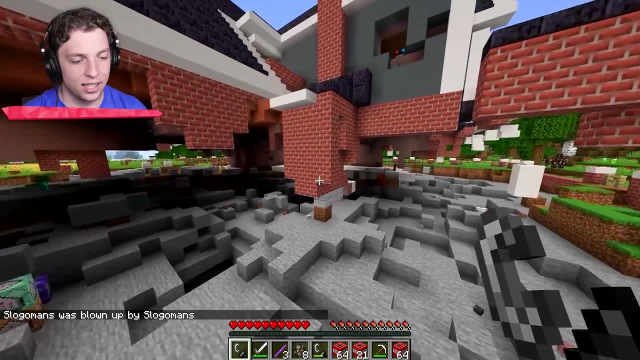 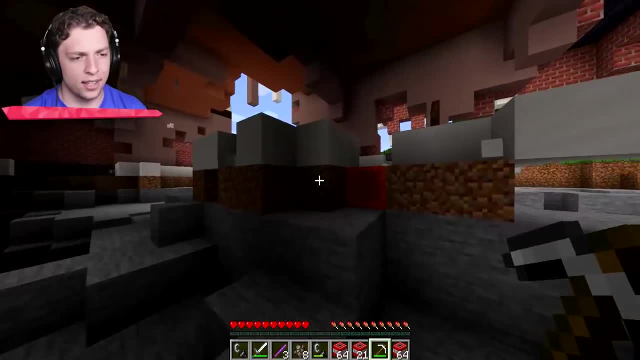 Okay, Okay, Nearly there, Now that we're just letting Josh do his thing, Like, how are you doing lately? Nearly there, Yeah, I'm actually really. Oh, we're nearly at full collapse. Couple more pieces and we are there. 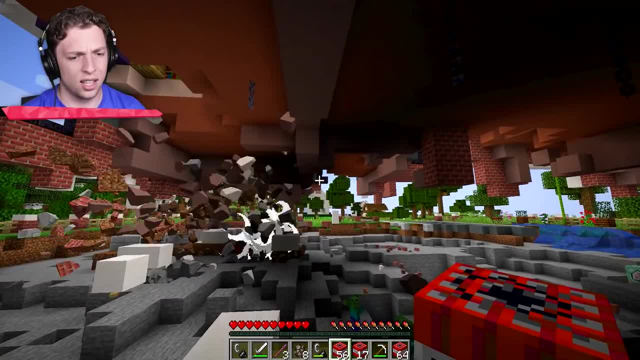 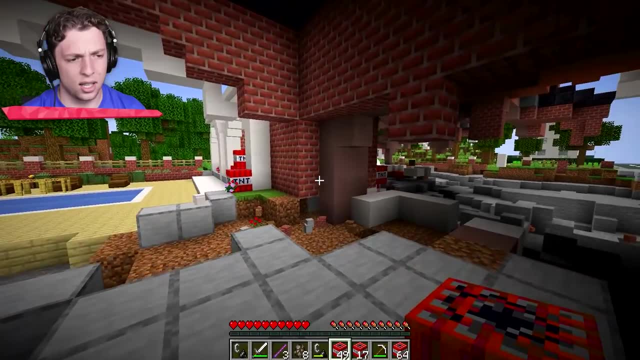 We're full destruction. You know what I did the other day? Yeah, tell me, I bought milk, Milk, Milk. What do you mean? what? Just a little bit of milk Crane. I know a fun challenge while we watch this. 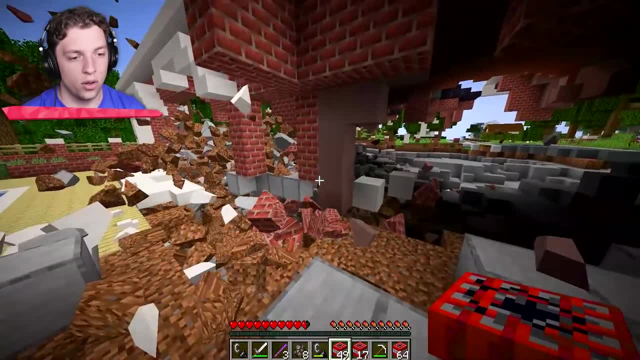 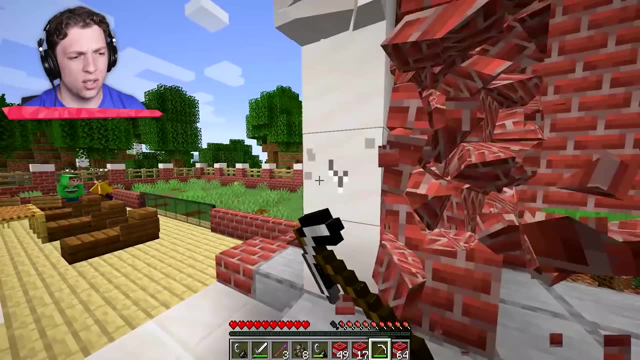 What, Oh Are you thinking what I'm thinking? The last couple of pieces, This whole thing comes down. Are you thinking what I'm thinking? More challenge, Word challenge, Word challenge, Word challenge. Okay, we invented this the other day. 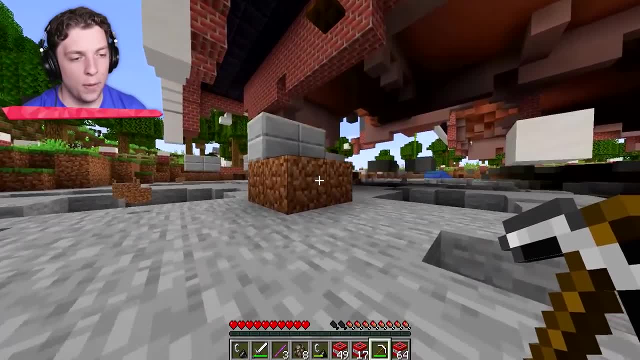 You start, You start Word, Word, start House. Okay, There's like one piece holding it together. Oh, no, Never mind, There's a few more: One, Two, Three, Four, Microphone. What are you guys doing? 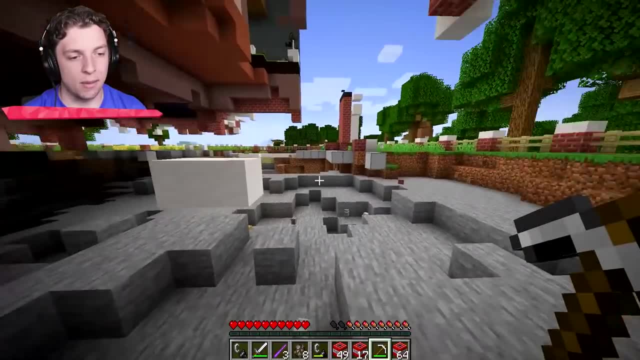 Okay, I'm not going to lie guys, The house is kind of floating in some parts Pants. We're letting you do the video and we're just doing a word challenge. Okay, Oh no, He's not letting us do the word challenge. 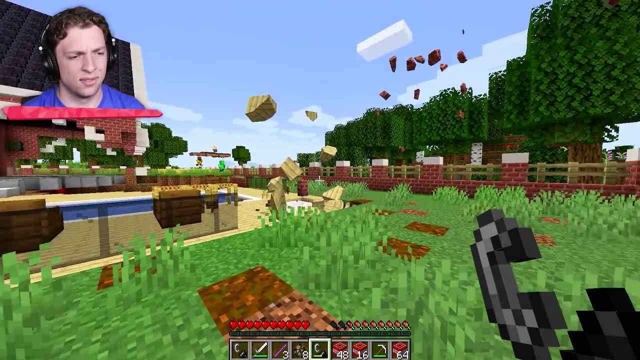 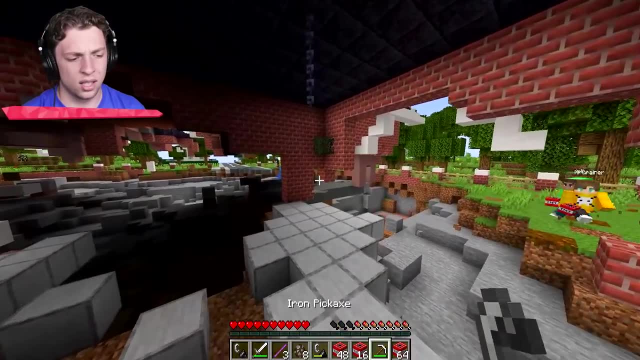 We'll do it another day. P&T. No, I did that already. You failed, You lost. Oh no, You lost the word challenge, Jess. Are you kidding me? Well, the house is pretty much floating now. Josh, the whole reason for us letting you do your thing was so you could let this house 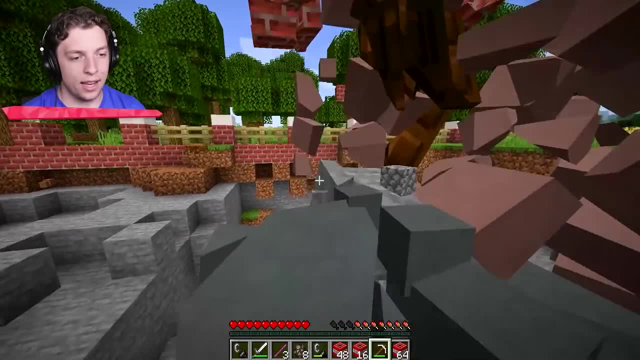 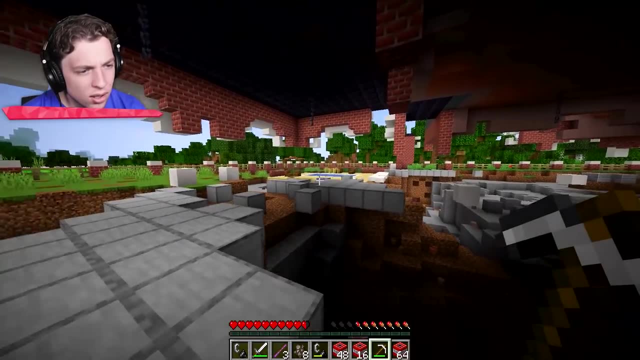 collapse and you failed. Well, yeah, It's not really doing what I tell it to do. He sounds more normal now. Are you back to normal, Josh? There must be a piece connected still, Well, no, Oh yeah. 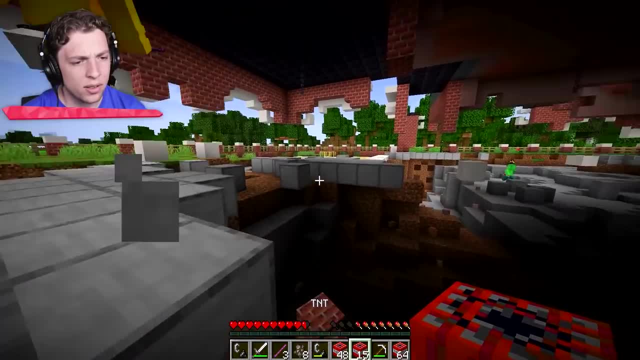 Yeah, I see it, I see it, I see it. Oh okay, Are you sure? Right here? Right here? No, it's not connected. Yeah, that one is Right over here, That's connected. We have to go up. 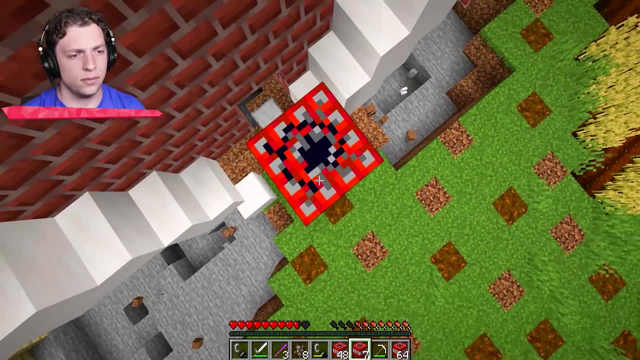 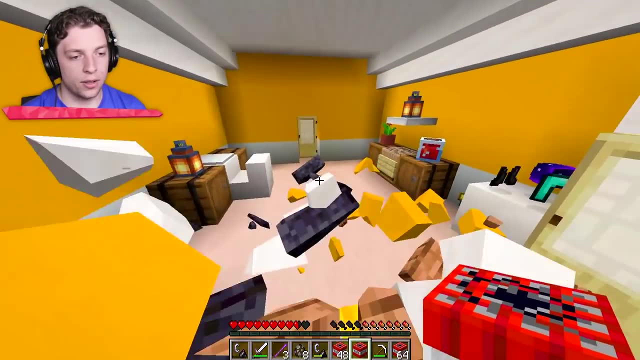 Oh, no, That's not connected. We must go higher. Which part? Okay, I don't think he's completely back to normal now. We must go higher. I mean, do we even help him, Jelly? No, Oh, the house is falling apart on the inside. 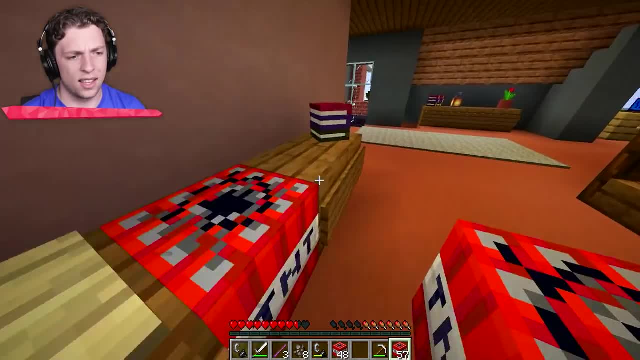 We can try the word challenge again, if you want. I don't really understand why it's not collapsing, to be honest, Yeah, Honestly, it's starting to upset me a bit. I think it's just like I fell through the roof. 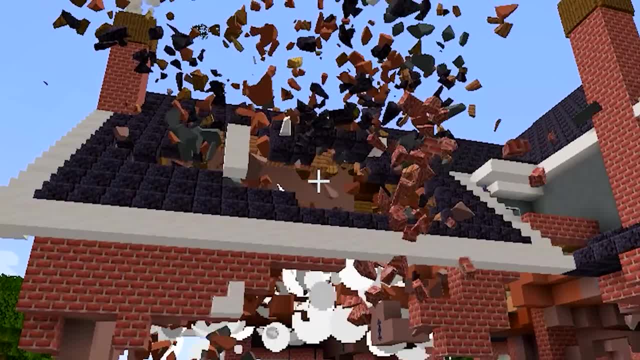 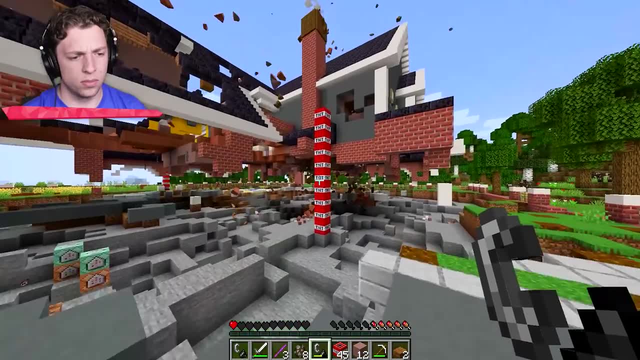 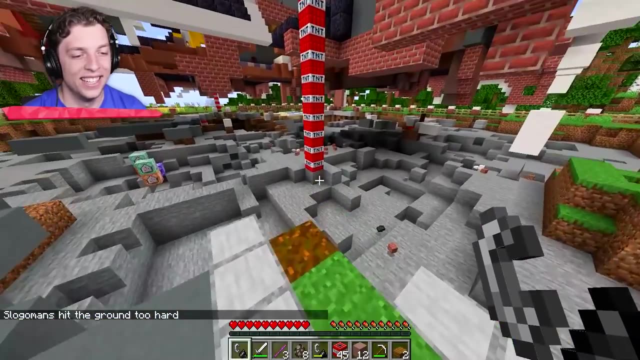 It's not all the way there. Whoa, Yes, Oh my God, Big boom, boom. It's still not falling, guys, Okay, You know what? Okay, Okay, Josh, you are allowed to go into creative and spam TNT everywhere, so you can get this out. 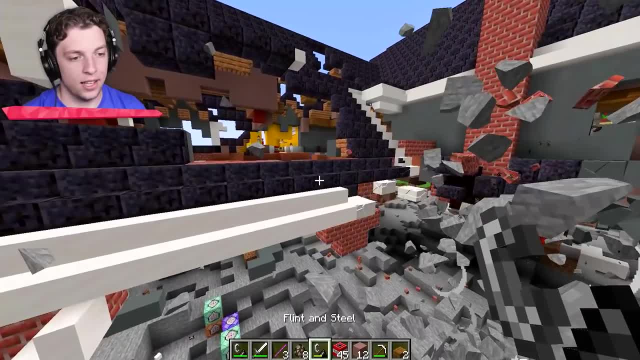 of your. Yeah, yeah, yeah, Thank you, It's allowed, Please. We want you to be done with this. okay, This is extremely. We want you to finish the house, please, Okay, Okay, Okay, I will do my duty. 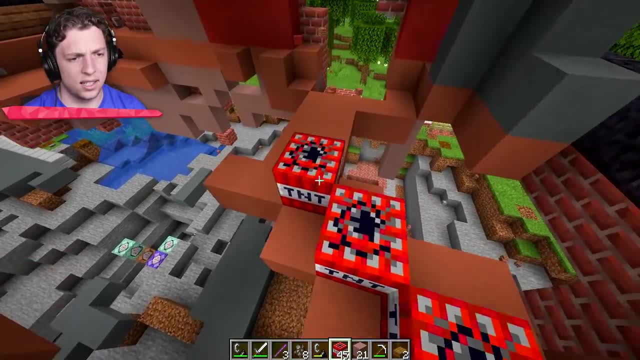 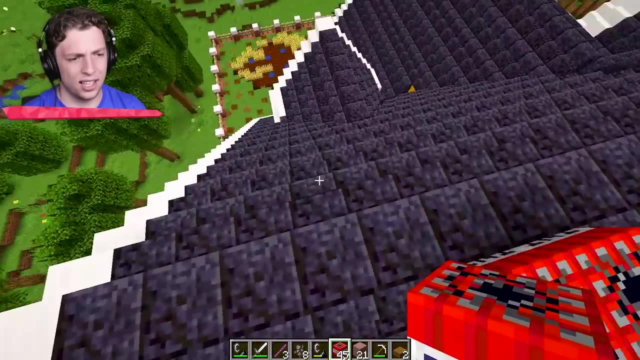 You know, this house is a lot bigger than I expected. actually, Josh is just recording his own video right now, And we'll put some on the roof as well. I suppose He's making a job really easy. Jelly, This is great. 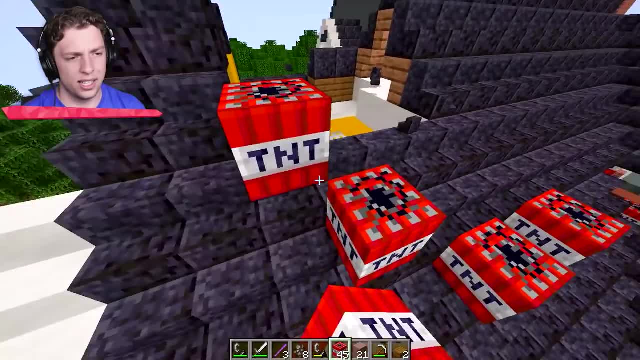 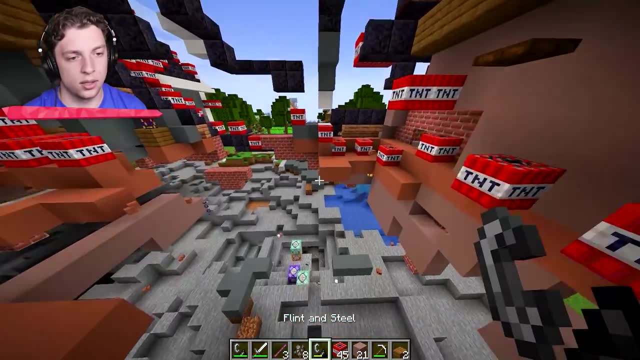 I don't really know what's wrong with this. We'll put some on the roof. Honestly, pretty much every inch is covered. If this doesn't blow up the whole thing, then, Josh, I think we should. I think we should leave it alone. 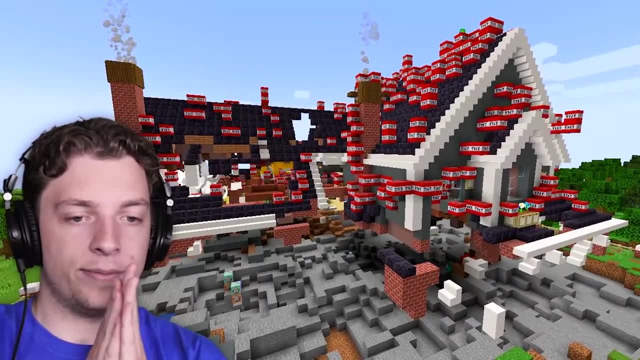 Okay, buddy, Yeah, Okay, bud. Are you ready to give up if this doesn't work? bud, Oh, is it going? Oh my God Jeez, Oh my God, Oh my God Beautiful. 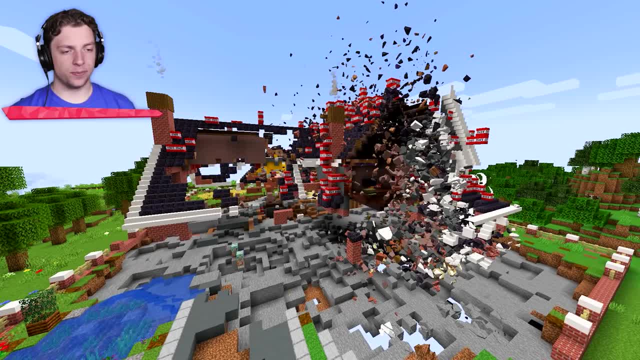 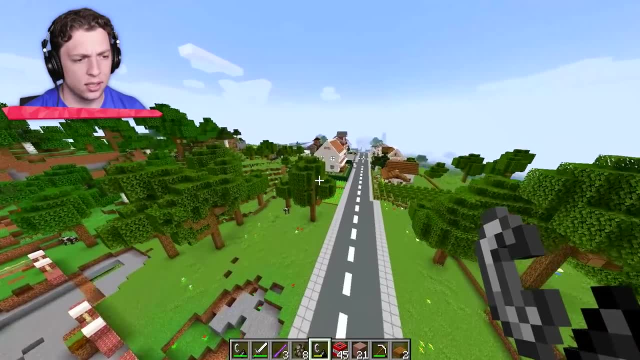 A lot of explosions, Absolutely beautiful. Oh, you're missing a little bit bud. I feel like we got most of it. I mean, yeah, I'm pretty satisfied with that. Oh, finally, I mean, but we've got the rest of the town to do. 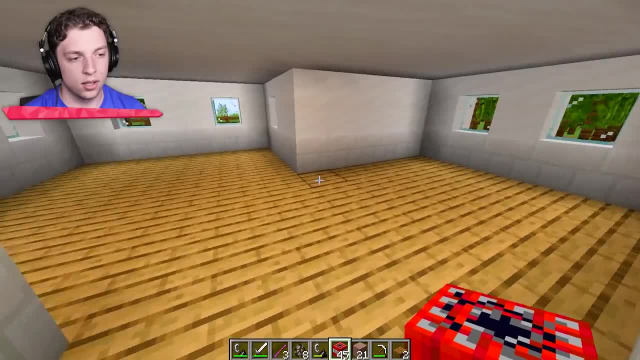 No, no, no, no, no, no, no. Josh, Josh, Josh, Josh, Josh, Yeah, Hey, hey, hey, hey, hey. Let's just deep breath real quick, But we've got so much more to explode. 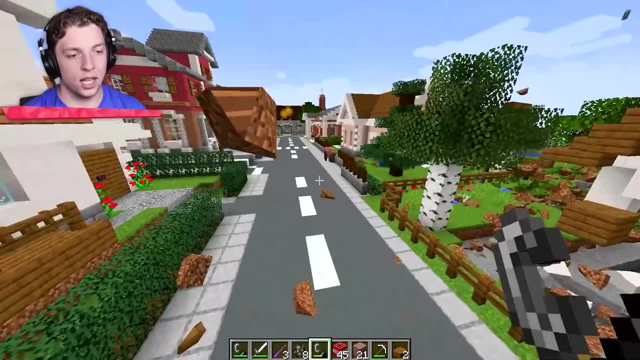 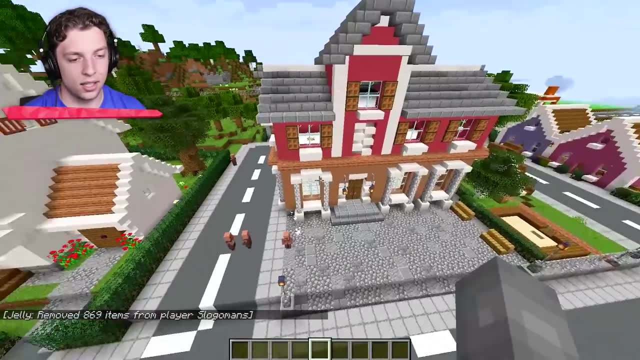 No, Josh, we will leave the neighbors alone. I just have to get going one house at a time and I can get this entire city gone. Jelly, I was fine with this when it was the house, but Hey, hey, don't clear my inventory. 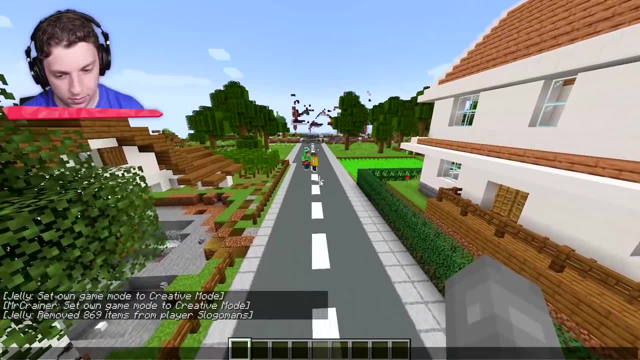 He's going to keep going forever. Jelly, We need to do something. We can't. We can't let you. We can't let you do this, Josh Slash. Oh, that's a good idea. He banned me, Wait.